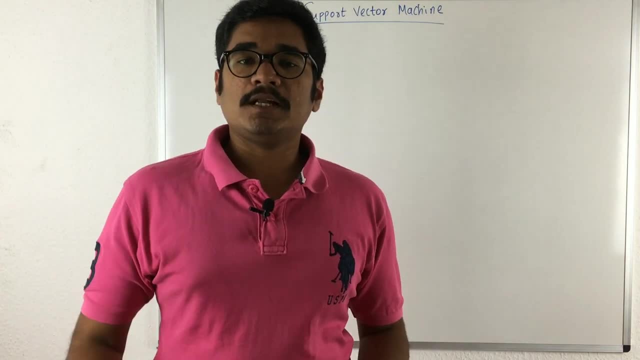 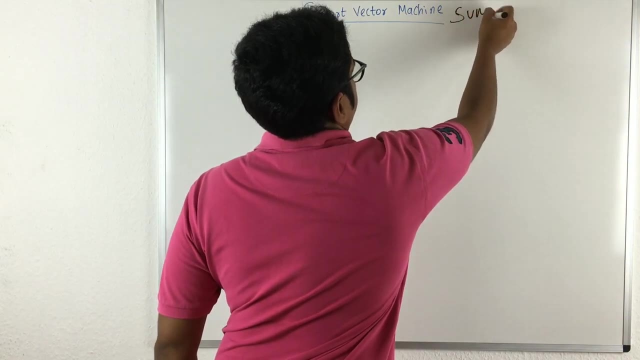 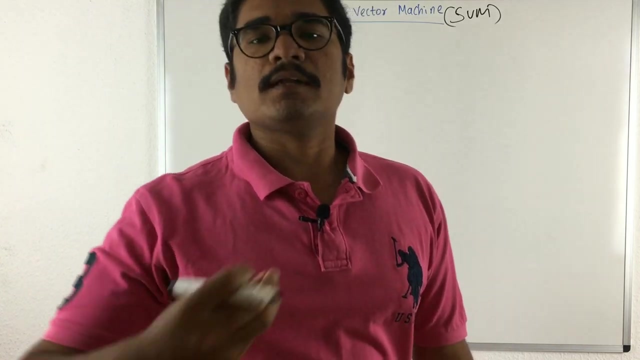 Hello people, welcome back to my channel. So today in this video, let's see another topic on machine learning, that is, we have the support vector machines, also called as SVM. So before we start with support vector machine, let's understand some of the applications where 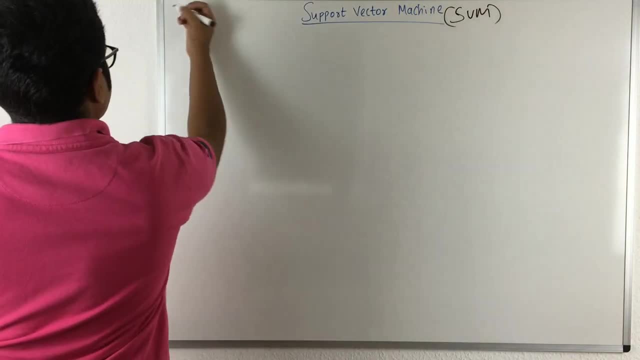 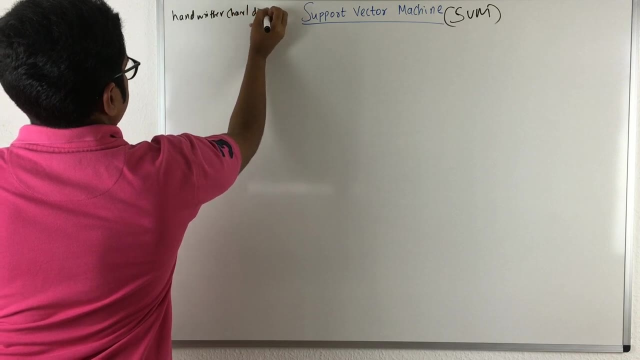 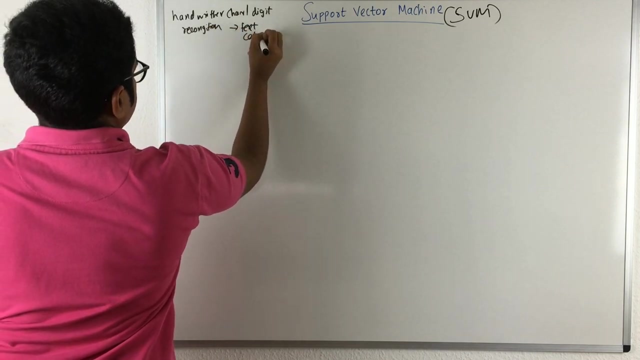 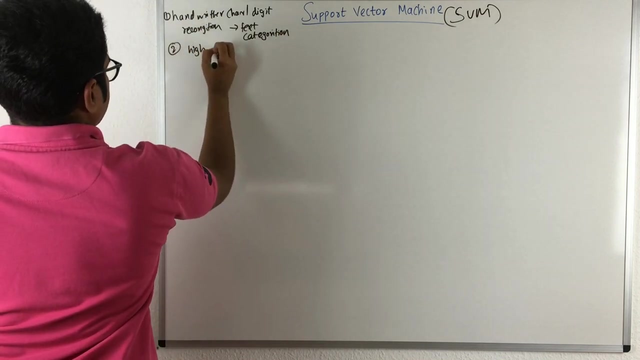 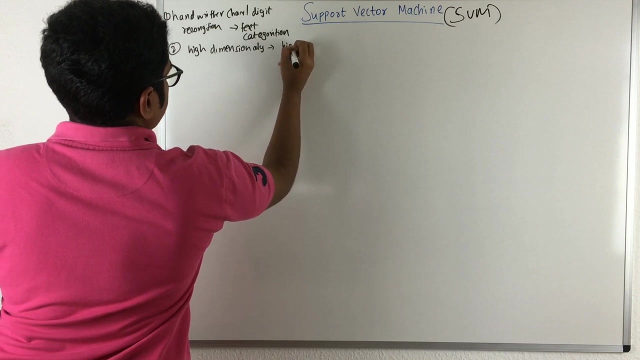 support vector machines are used, So it's used in applications ranging from handwritten character or digit recognition To you have something called as text categorization. Also, SVMs perform very well on high dimensional data, And thus it solves the problem of high dimensionality. 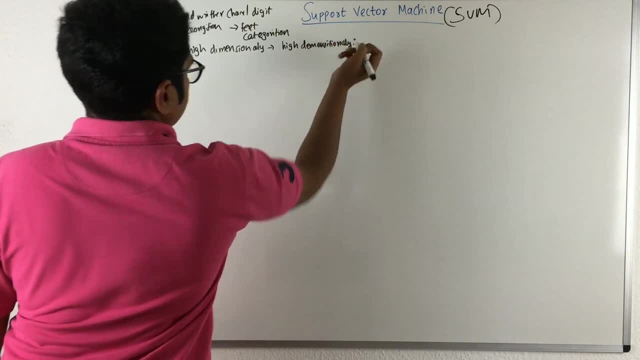 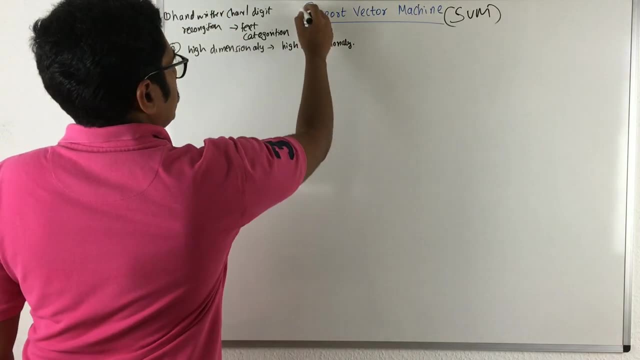 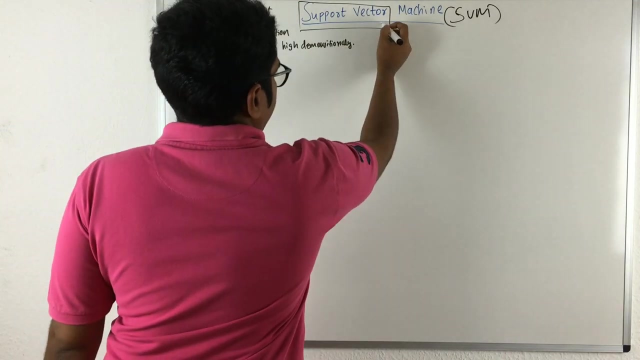 That is the problem with many of the other classifiers. So SVM performs well with high dimensional data as well. Now there is one thing, that is, you have this two terms called as support and vector, Now what this basically means. So vector in machine learning means data or examples. 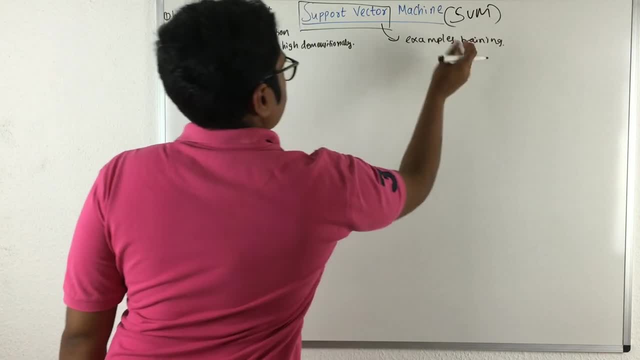 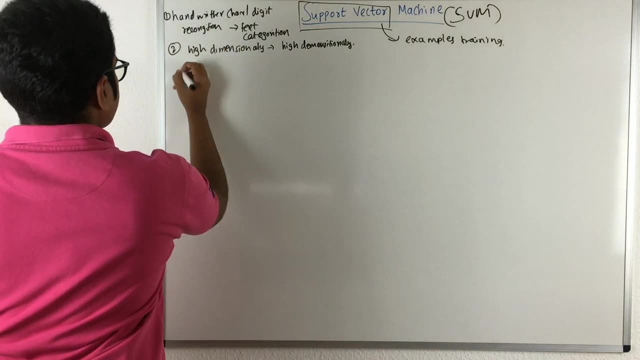 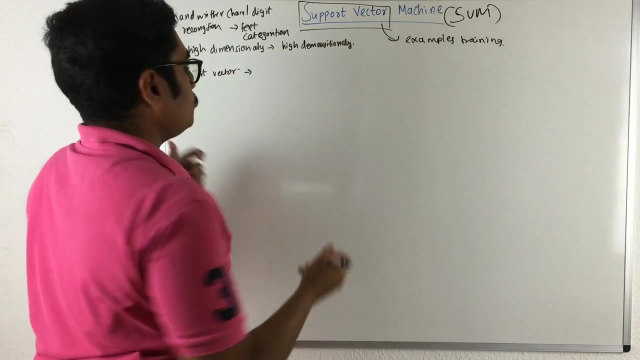 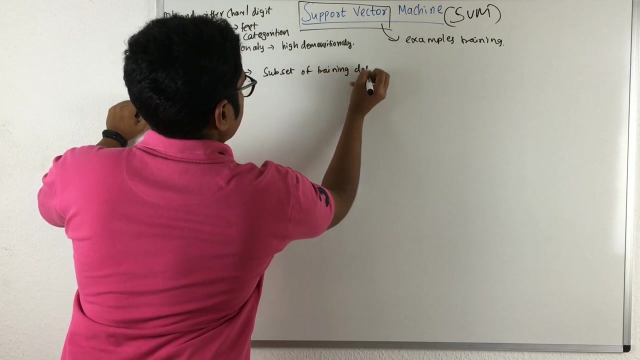 or the training examples means the. with the help of training examples, you construct some machine or classifier. so it's simple as that. so support vector SVMs, areugold, support vector machine, both or design respectively. So in this example, In SVM, you use the subset of training data and it is used to represent your decision. 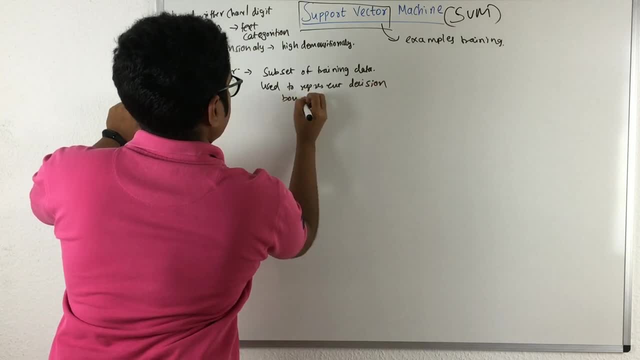 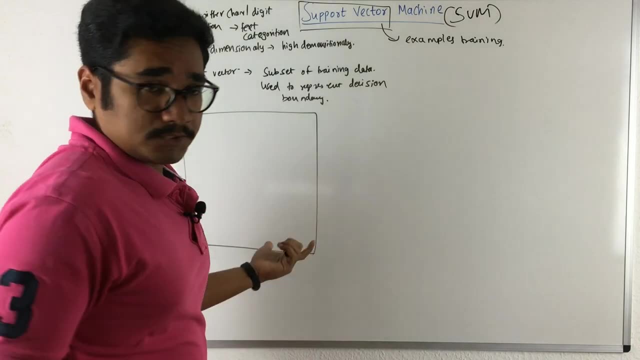 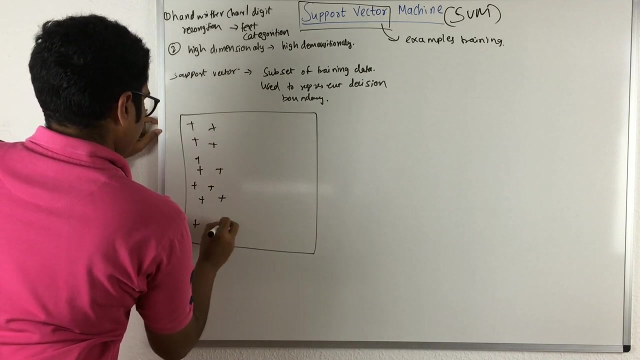 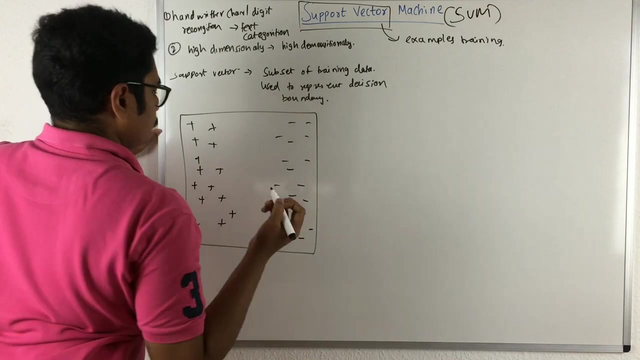 boundary. So you have something like this: So this will be our decision boundary- and say you have some instances- positive instances- to the left hand side, and you have negative instances or negative classes. So this is a just a random data set that I have considered. now you can have something. 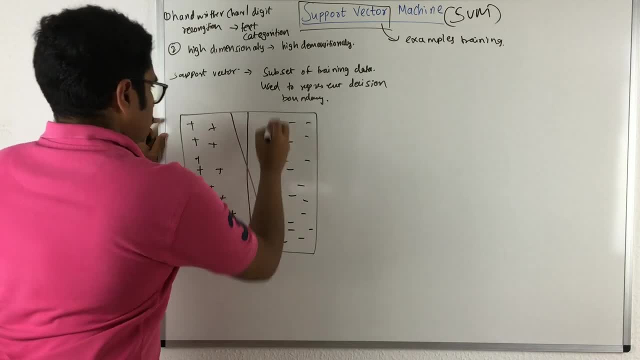 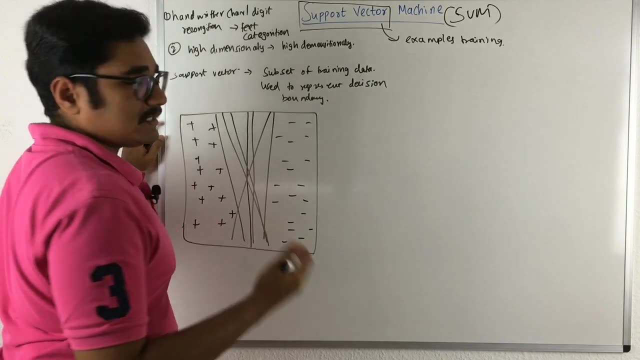 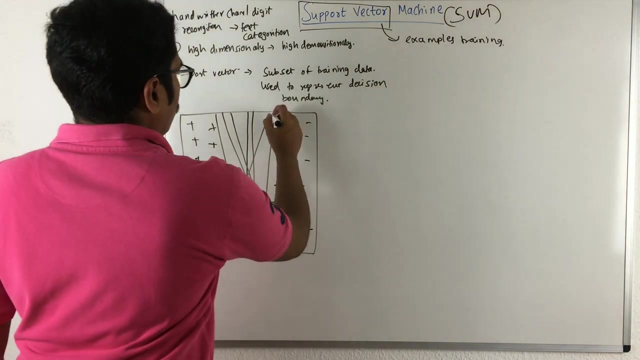 like this and you have some lines, So these are basically hyper planes. So this are used to separate this data set for being classified as positive and negative instances. Now there is one important thing in SVM That you need to remember: that it all works on the concept of something called as maximal. 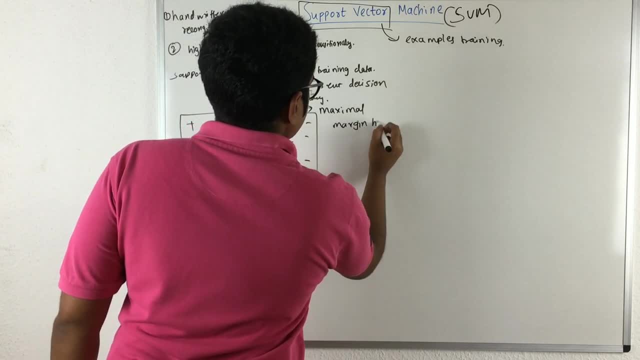 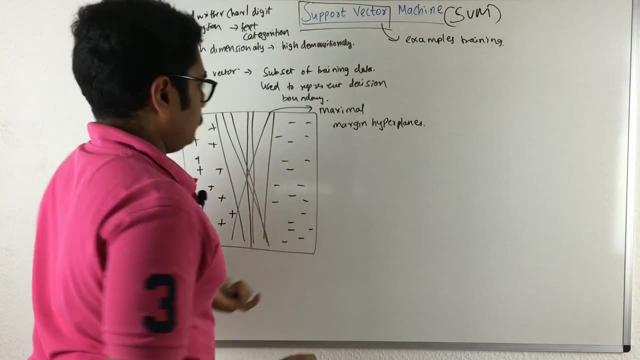 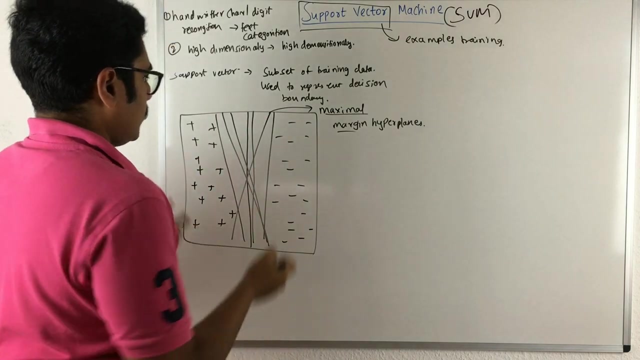 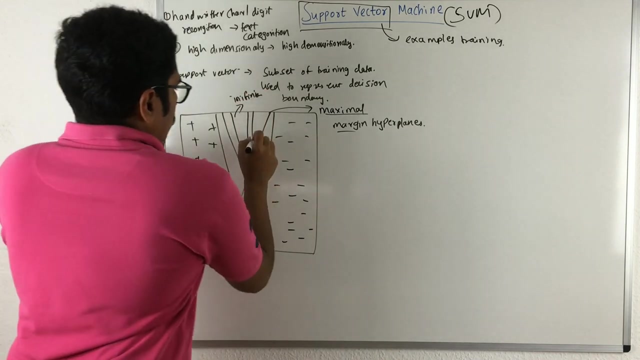 margin: hyper planes. So this what I've drawn is called as an hyper plane. Now, what is maximal margin? now, before that, just consider three things on this line. So this things or this lines can be infinite in number. Okay, Okay, Okay. 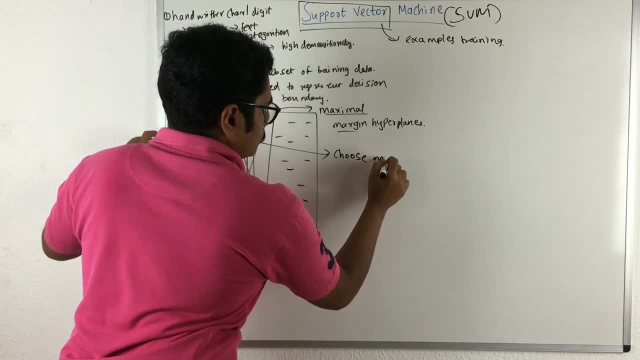 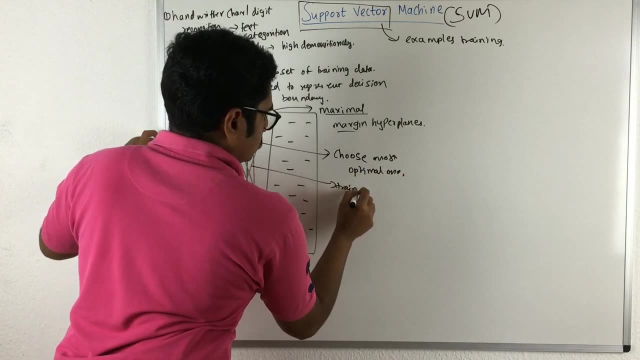 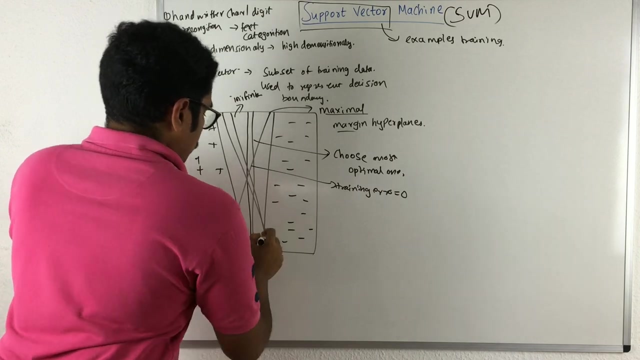 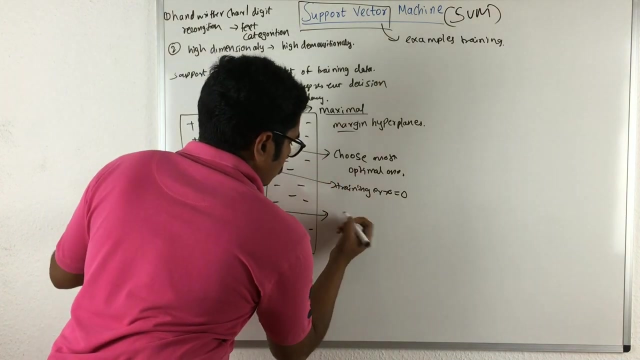 Now you need to choose any one of them. which is the most optimal. choose most optimal one, Then the training errors on this is zero. Now there is a case where you need to choose any of this one hyper plane. So in that the chosen hyper plane may not perform well in future, or like it's not, 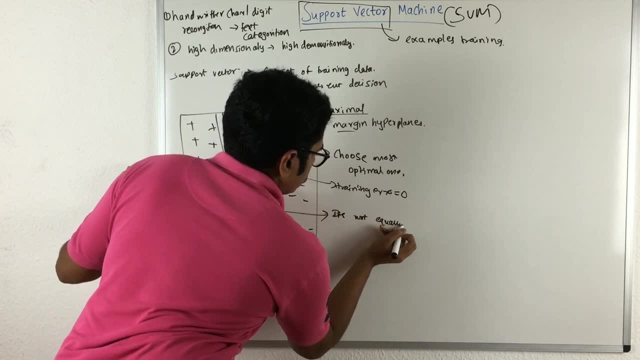 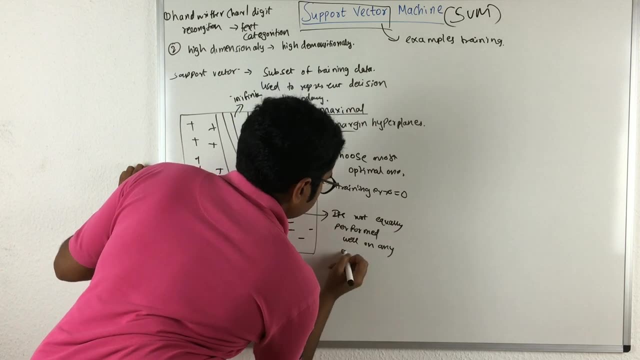 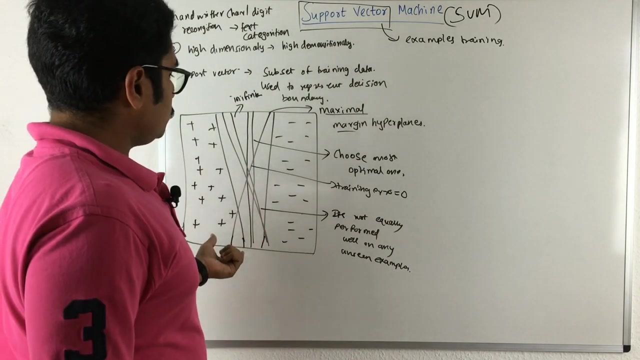 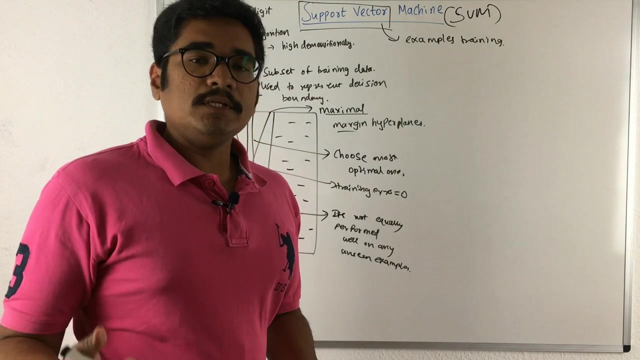 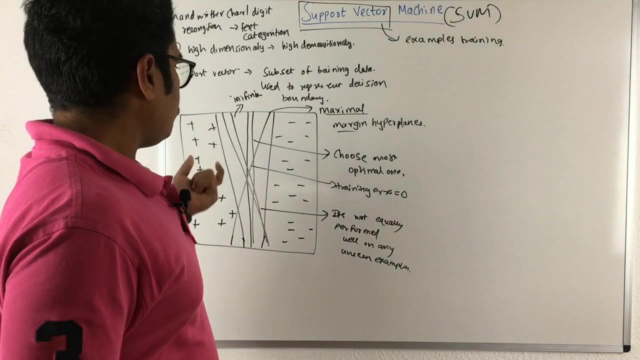 Equally performed well on any unseen examples means now, at this moment, suppose you chosen one hyper plane and if you tomorrow use that hyper plane for any other classification, then it cannot equally separate all the unseen or future instances. So that is the Major drawback of this. so that means you need to choose this hyper planes very carefully. 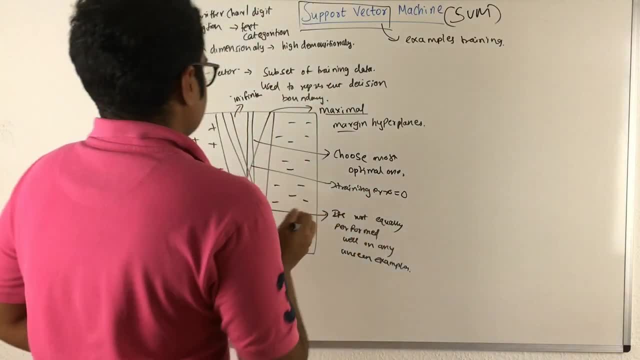 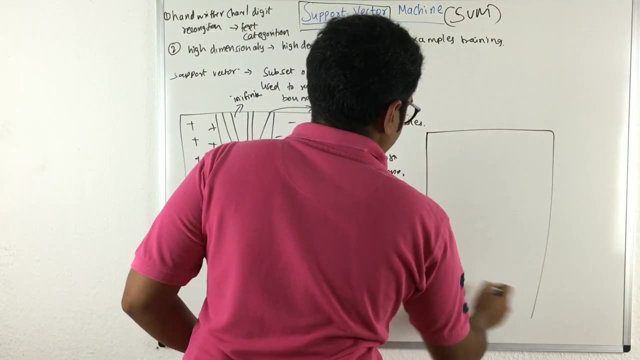 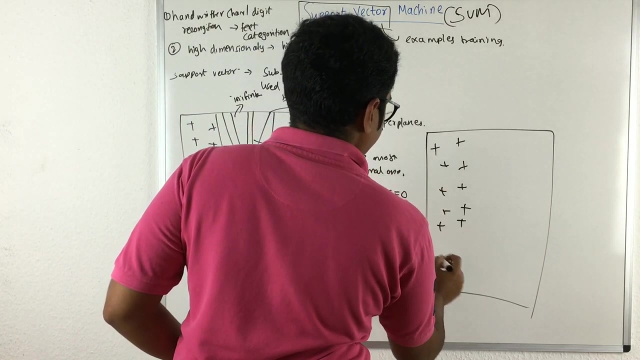 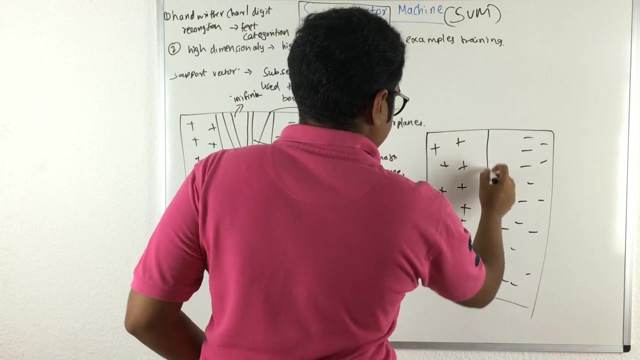 when you construct any linear SVM. So one main thing, just to understand the concept of how you choose this hyper planes, just consider this decision boundary. You have the same instances- positive, Same negative instances- And see, I just take one of this just to show you how this decision boundary or this hyper plane, 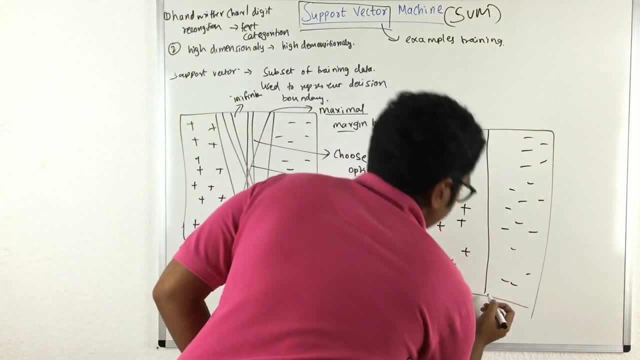 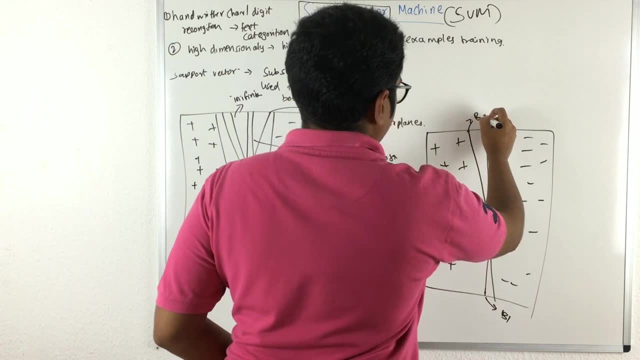 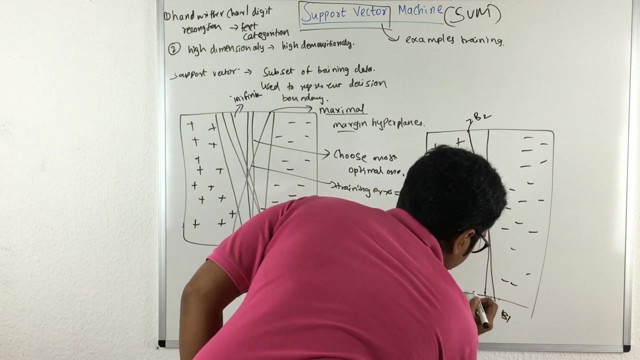 affects your performance of linear SVM. So this is one boundary, say this is boundary one and you just have another boundary, This is boundary two. and let's say there is some area which has been spanned by this boundary one, just to show that this area is owned by B1, or first boundary. 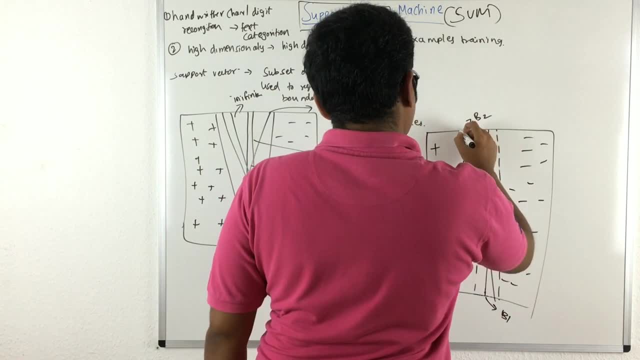 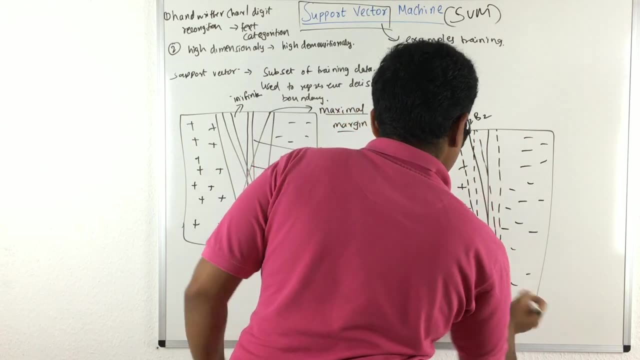 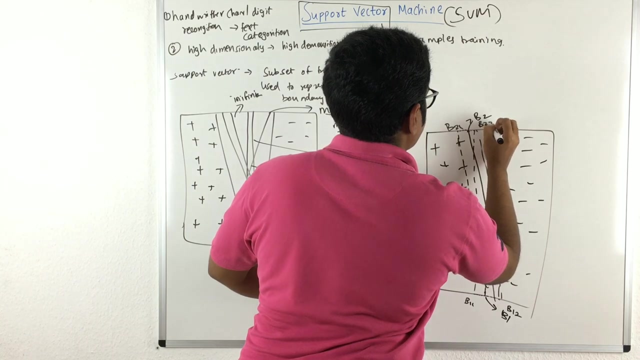 Okay. Similarly, you have some area span on the left side, some on the right side, So it is something like this: Just label this as B 1 1 and B 1- 2, and this has B 2 1 and B 2- 2. now you can see the gap. 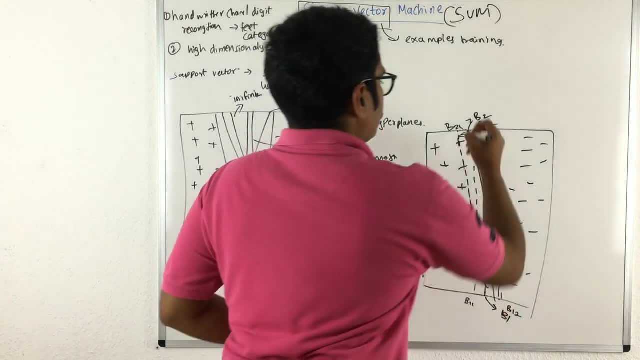 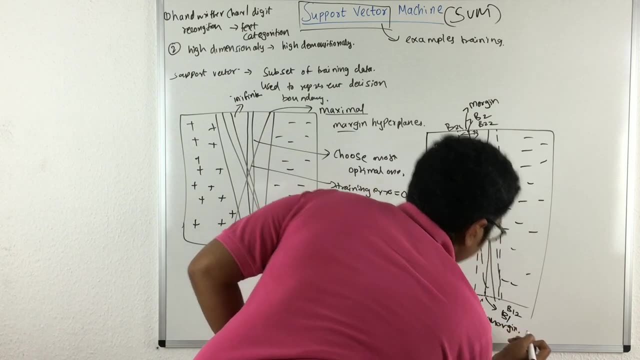 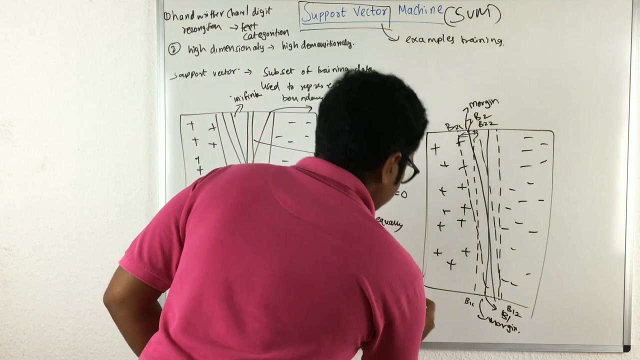 between these two boundaries set by left and right. So these are called as margins, And here also you have margin. So what do you basically see? Choosing your hyper plane is that if your margin is higher than you go with that hyper plane. So here, in this case, the margin of hyper plane B1 is greater than margin of hyper plane B2.. 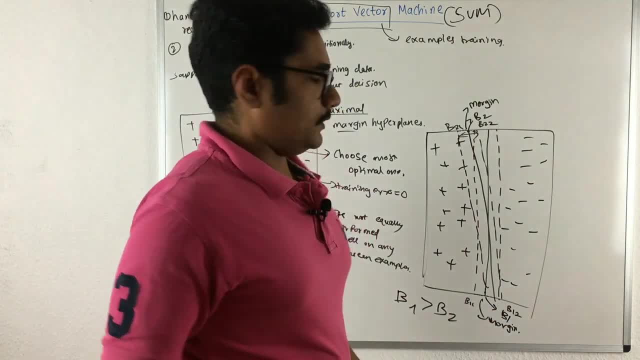 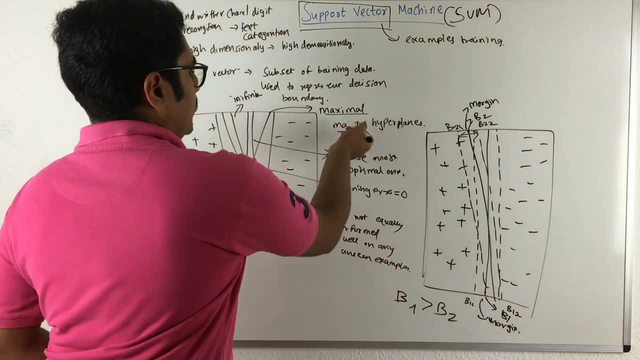 So you just consider B1 and you go for that for classification. So that is the main idea of choosing the marginal hyper plane. So that's where the name maximal margin hyper planes comes into picture. Now there are two cases of this, like if you choose your, 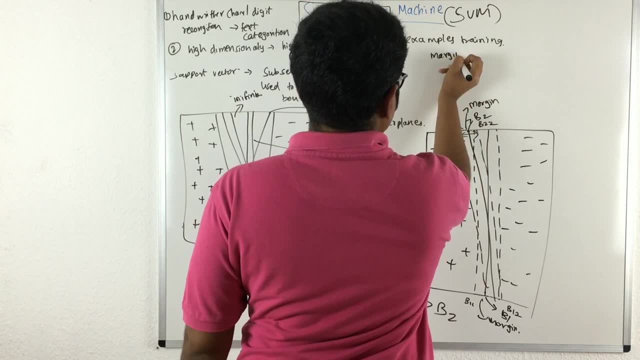 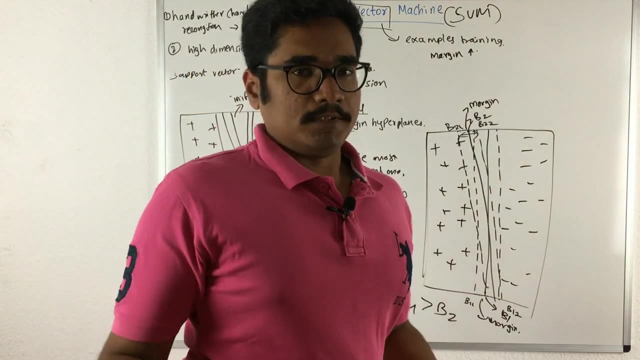 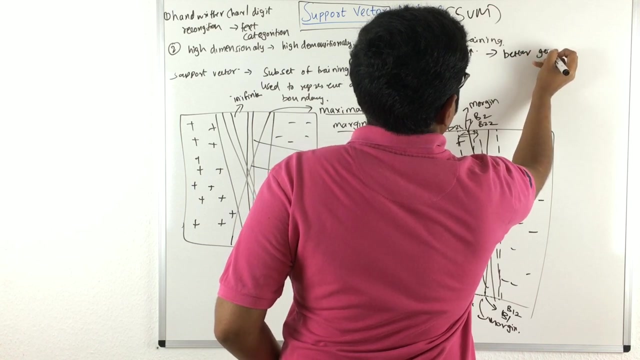 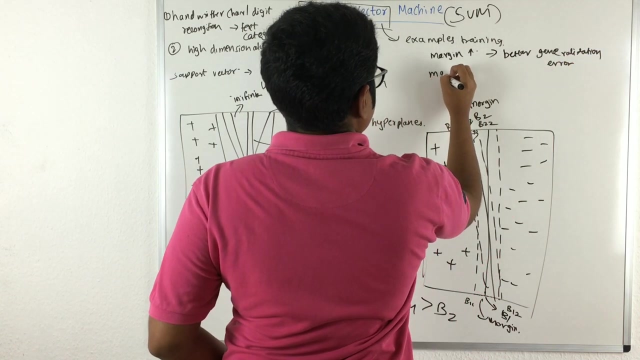 Margin. And if your margin is higher means why it's always called, or what is the reason behind choosing highest margin, hyper plane. So if your margin is higher, that means you have better control over your generalization error, as if you go with lesser margin, then your model will fall a victim of. 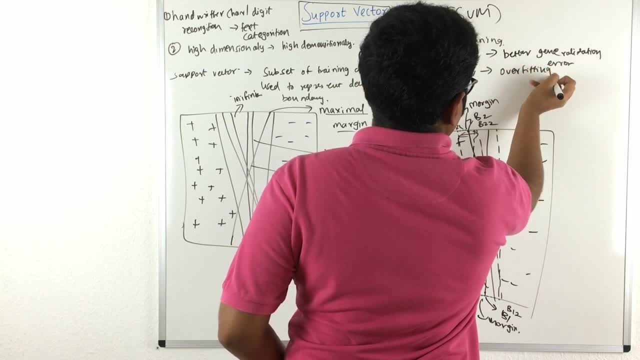 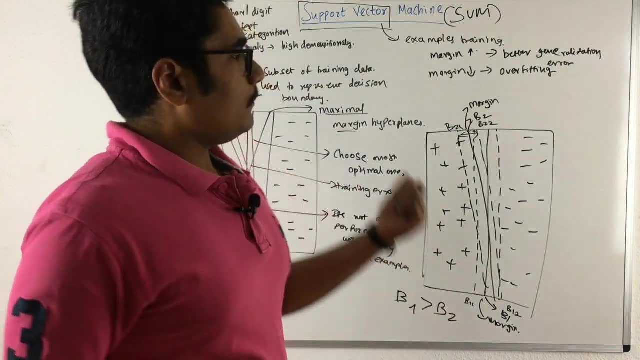 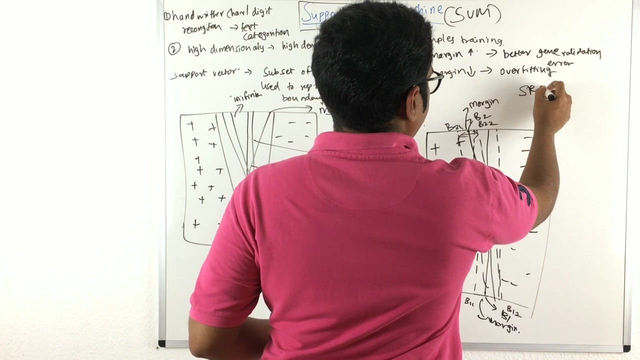 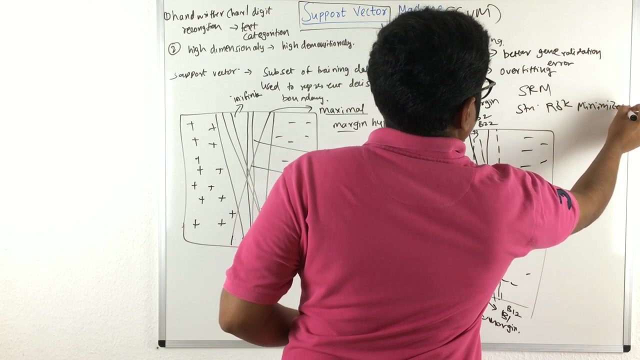 Overfitting. So that is a problem we have discussed in decision trees, So similar case can happen to SVM as well. Now this: whatever concept which I spoke right now in statistics It is called something as SRM, that is, structural risk minimization. 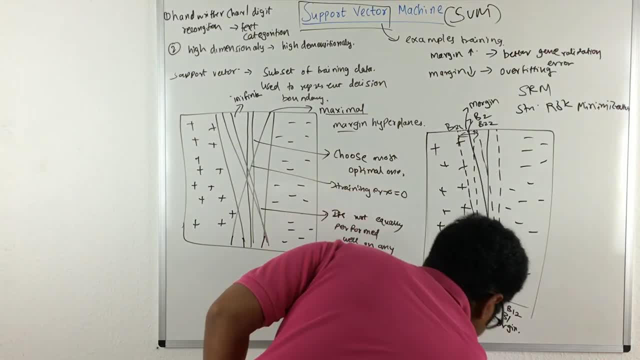 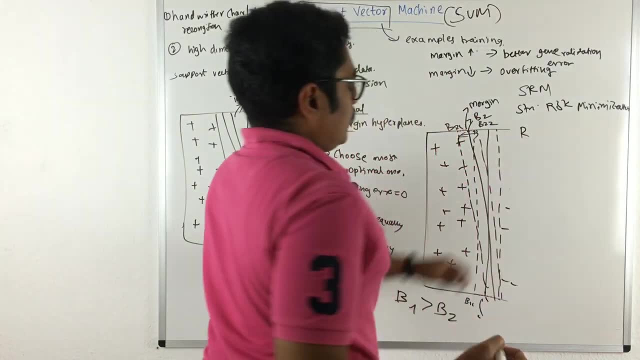 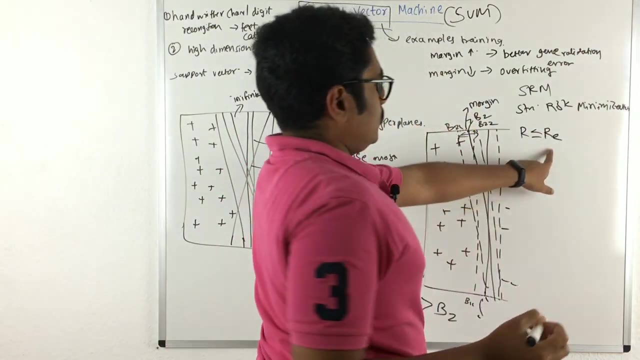 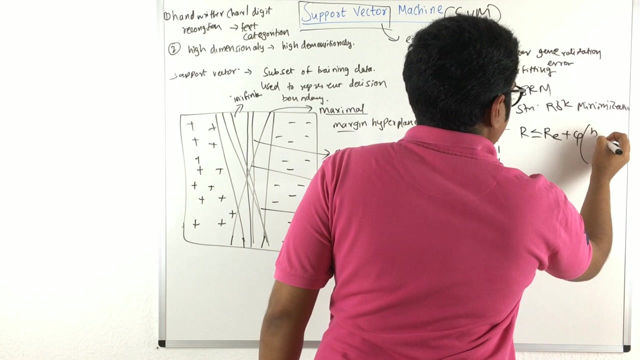 So in that for any classifier you have the equation. So for any classifier that is for our, you estimate that is an inequality equation. It is. you have the, that is the training error. re plus, you have some monotone increasing function and it is given over H, that is capacity divided by total number of training. examples: